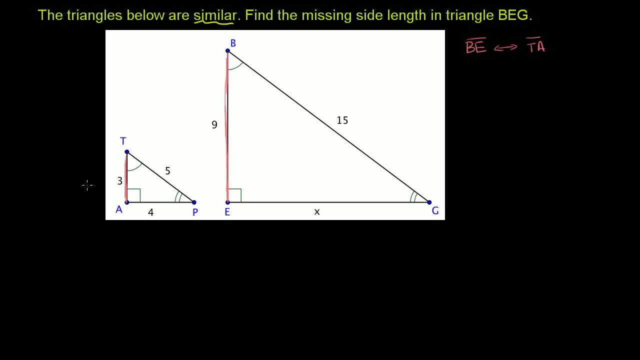 and these sides are the ones in between them. We also know that side EX, which is the one that we have to figure out the length of. we also know that side EX right over here, or actually I should say EG. we know that side EG over here. 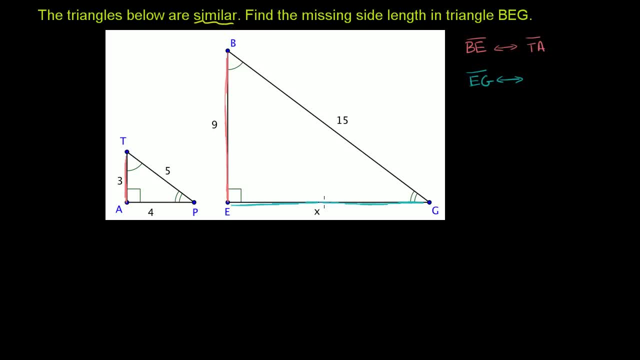 corresponds to it's between the right angle and the double arc angle, between the right angle and the double arc angle. it corresponds to side AP. It corresponds to side AP And we know from similar triangles that the ratio between corresponding sides has to be the same. 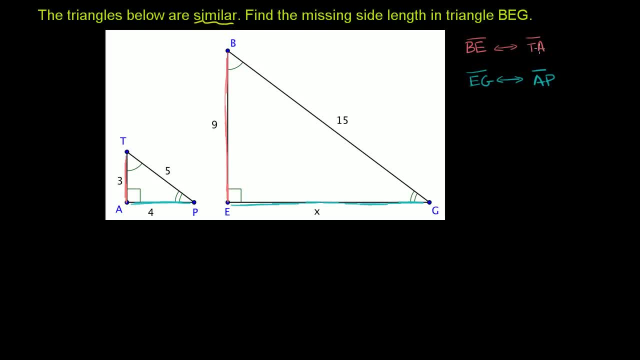 So, for example, the ratio between BE and TA has to be the same as the ratio between EG and AP. So let's write that down, The ratio between BE, and let me write it down here actually, so I have a little bit more space. 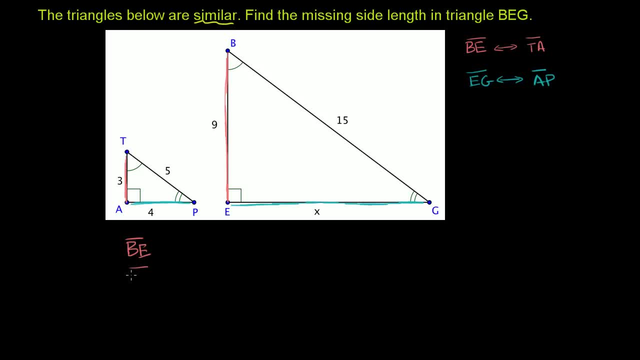 The ratio between segment BE and segment TA has to be equal to the ratio between segment. let me do that in blue- between segment EG and segment AP, And we know the length of BE. We know that that is equal to 9.. This is equal to 9.. 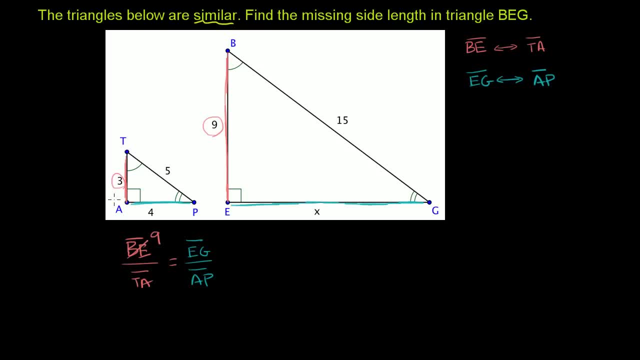 They give us that right over here, Right over there, And we know that TA is equal to 3.. This is equal to 3.. So 9 over 3 has got to be equal to EG over AP, And we also know what AP is. 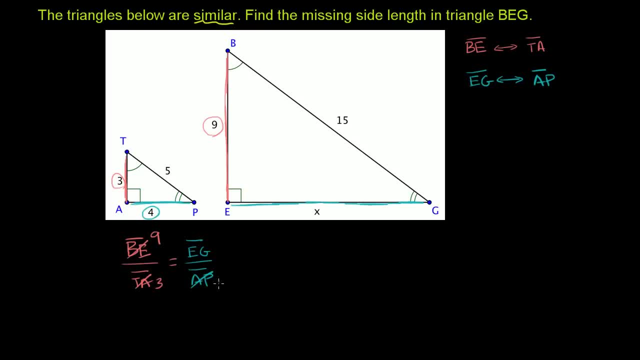 AP they give us right over. there is length 4.. So this boils down to 9 divided by 3, which is just 3, must be equal to EG. Well, an EG actually, let's just call that X. 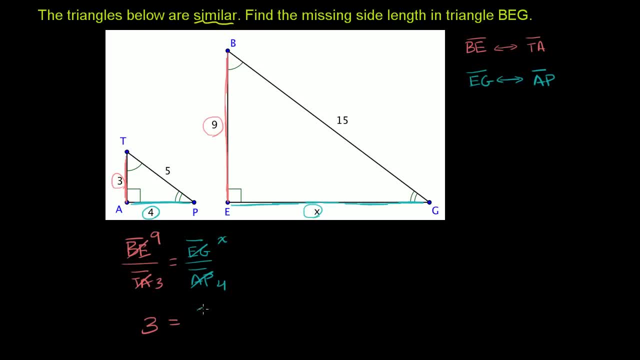 Since they call it X, this is going to be equal to X. It is equal to AP, X over 4.. EG is X, AP is 4.. And to solve this for X, you just have to multiply both sides by 4.. 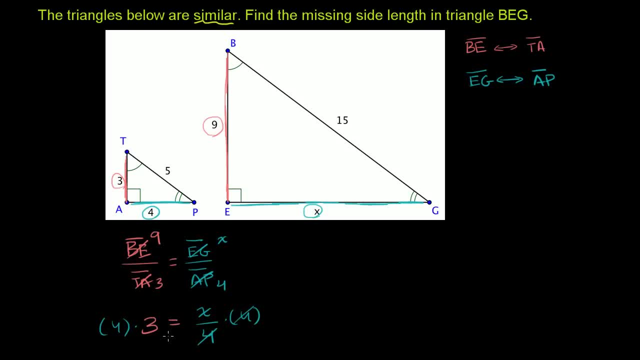 You multiply both sides by 4.. These 4's cancel out. This becomes 12.. So you get: X must be equal to 12, which is the missing length on this triangle right over here.